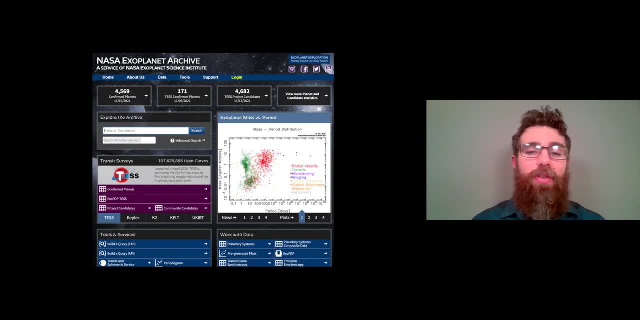 If you go to the exoplanet archive you get lots of plots that give you the radiuses of the exoplanets, the masses, the orbital period, things like that. This has all of the current known information about exoplanets, as well as candidates, And you can generate plots that. 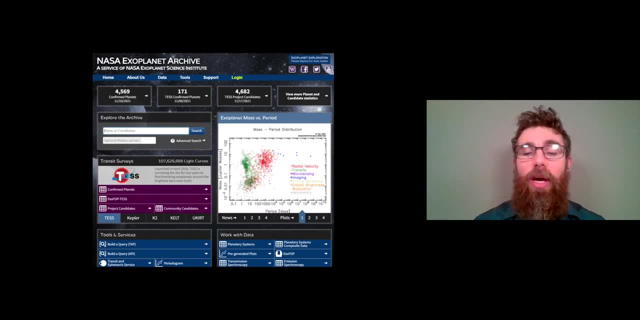 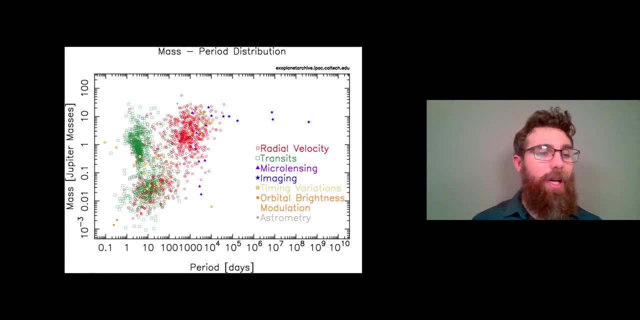 are already made. So you've got pre-generated plots at the bottom or you can have a look at the data and create your own plots, And when we do that we've got orbital period against the mass of the planet in Jupiter masses And you've got quite a range there. 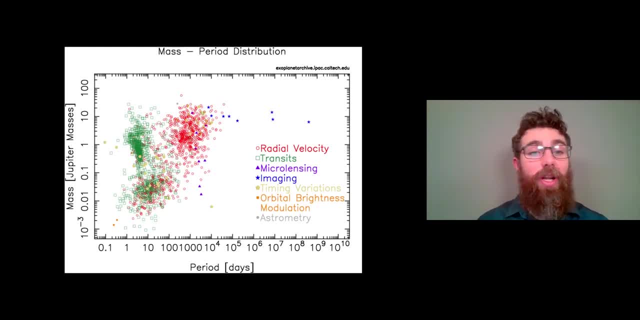 But note that a lot of your planets are green, which is the transit method again, And they're also to the left and upper part of the plot, which basically means large planets close to their stars are easy to find, for obvious reasons, And then we can do the orbital period against the 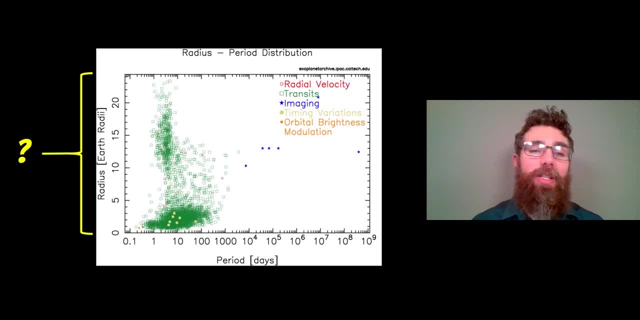 radius of the actual exoplanet. But how do we actually get that radius? And that's what we're going to have a look at in a minute. So we've got the orbital period and then we have the radius, and we can check out the orbital period in another video. So it's fairly straightforward. So we have. 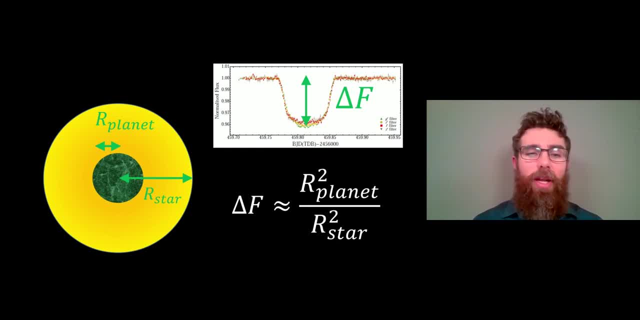 the radius of the star and the radius of the planet, And it's basically just the area of those subtractions And whatever you're left over with, or that's how we could basically get the radius of the exoplanet. So on the equation there you've got delta f, which is your change in flux, or 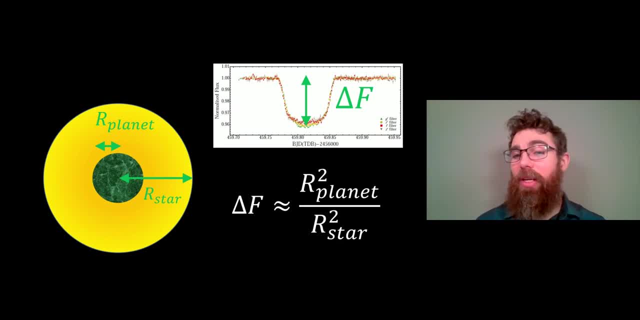 brightness of the star. So if the star dims down by three percent, then that is going to be our delta f, which would be 0.03.. And that would equal the square, the radius of the exoplanet over the square of the radius of the star. And we can rearrange that. 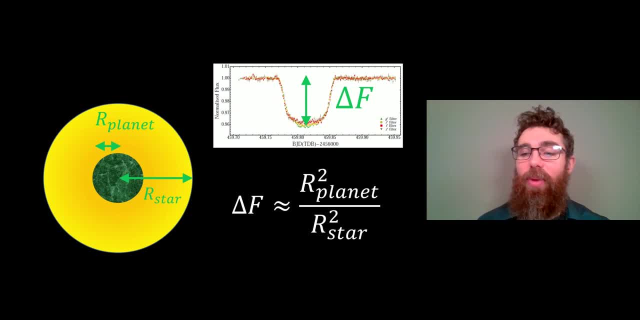 for the radius of the planet. And there we are: We have the radius of the planet, But I should note that we need- we do need to have the radius of the star in order to do that, But the radius of the star can be calculated using other methods. So, a lot of the time, 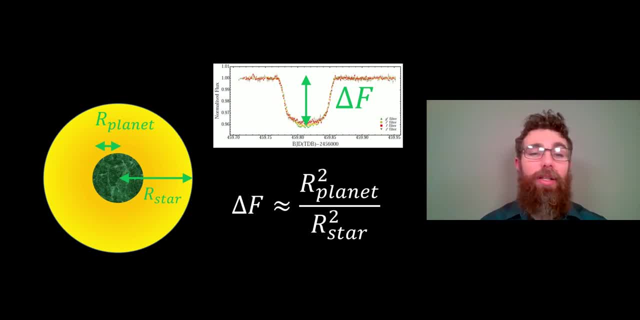 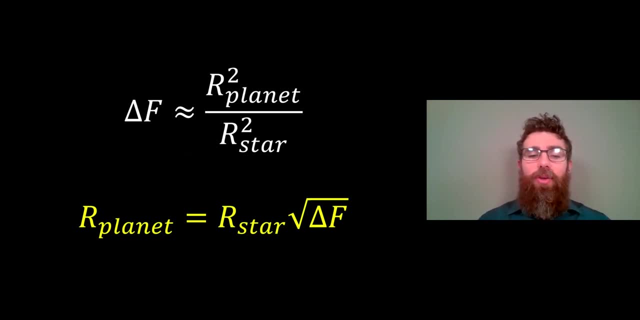 that information would already be available once you've detected a planet. So if we rearrange for the radius of the planet, we get this at the bottom here. So your radius of the planet is equal to the radius of the star times, the square root of the change in